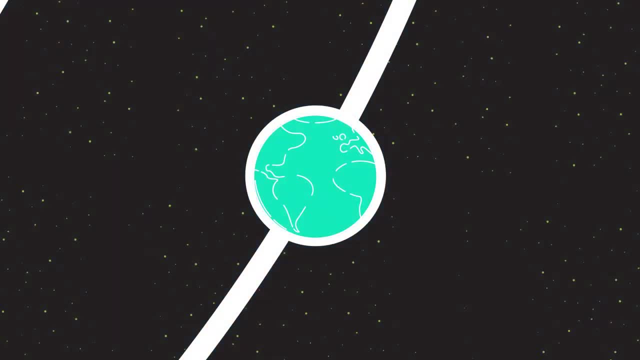 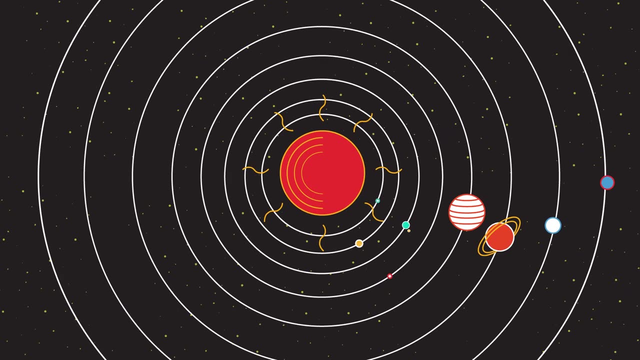 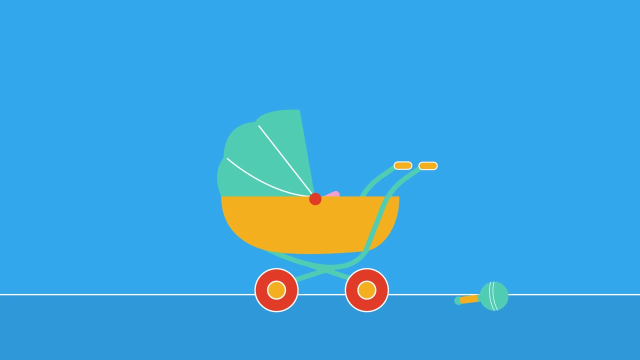 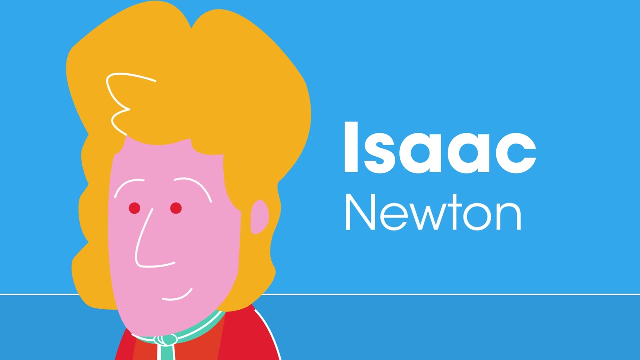 by gravity. Without the gravitational force, there would be no moons orbiting planets, no planets orbiting stars and no stars held in galaxies. It's something we discover as babies and we take it for granted. Famously, the concept of gravity was first proposed by Isaac Newton in the 1680s in his 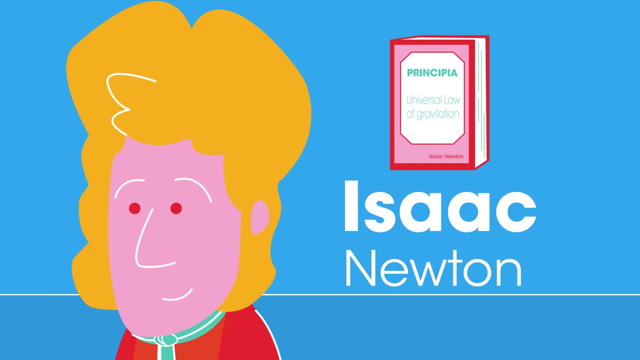 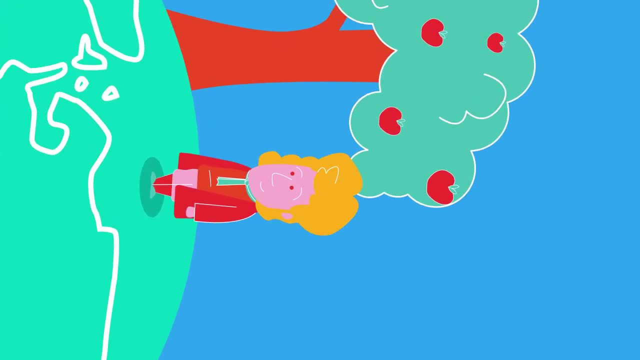 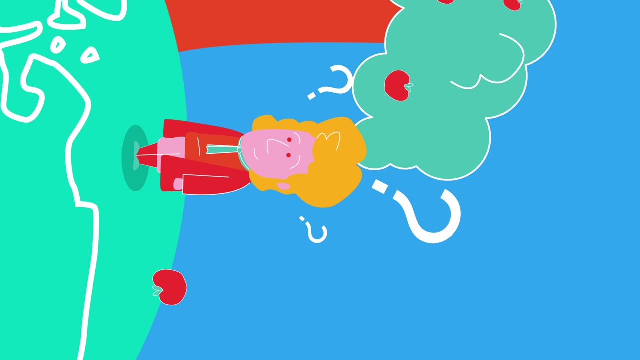 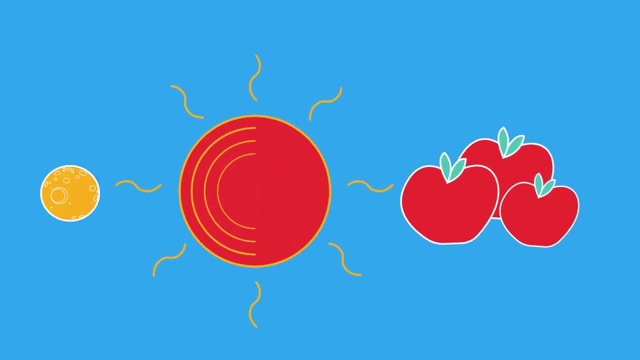 book Principia, which contained the universal law of gravitation. As the legend goes, he was sitting under an apple tree when an apple fell on his head and he began wondering what pulled it to the ground. Newton had the idea that gravity acted not just on apples, but also the sun. the moon. 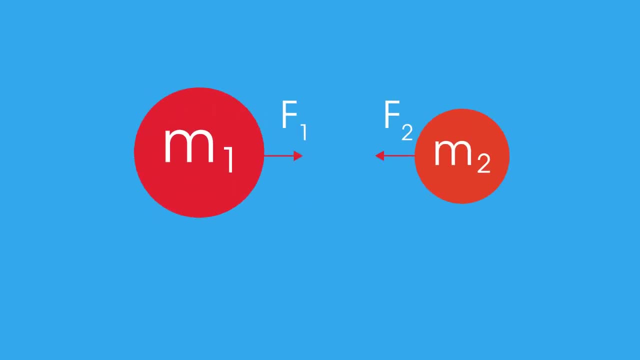 and the planets. The force increases as either or both of the masses- m1 and m2- increase and drops off by the square of the distance r between them. So, for example, doubling the mass of one of the objects also doubles the force of gravity. 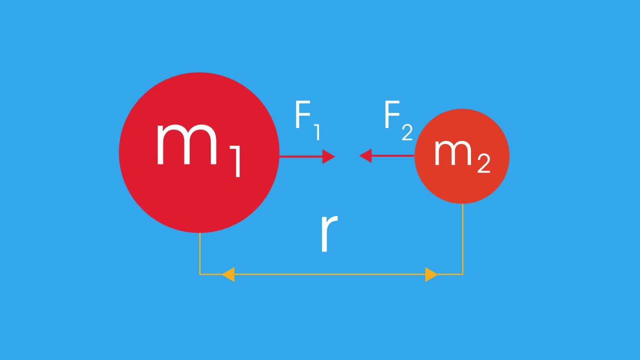 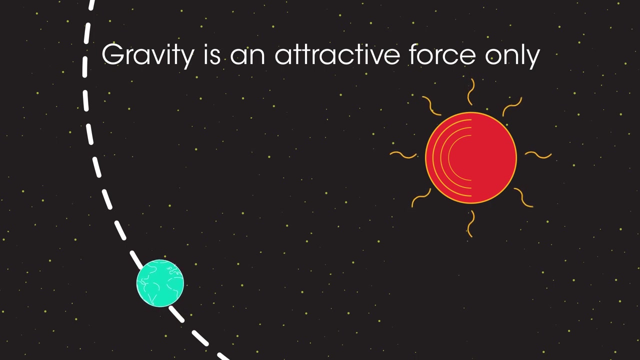 experienced. But doubling the distance between the two objects results in the force being reduced to one quarter of the original value. Gravity is an attractive force only and acts weaker over long distances. Gravity is an attractive force only and acts weaker over long distances. 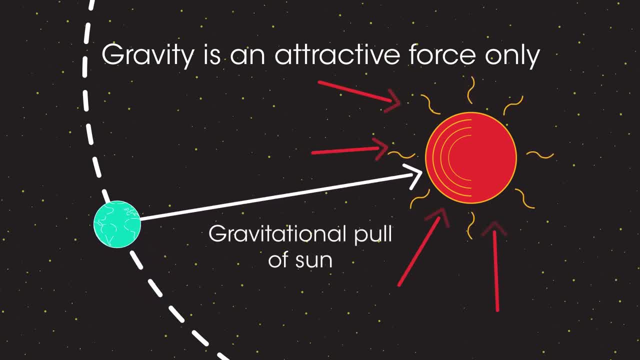 It's the gravitational force between two objects. It's the gravitational force between two objects. It's the gravitational force between the Earth and the Sun which keeps the Earth in orbit. Without this force, the Earth would continue to travel in a straight line. 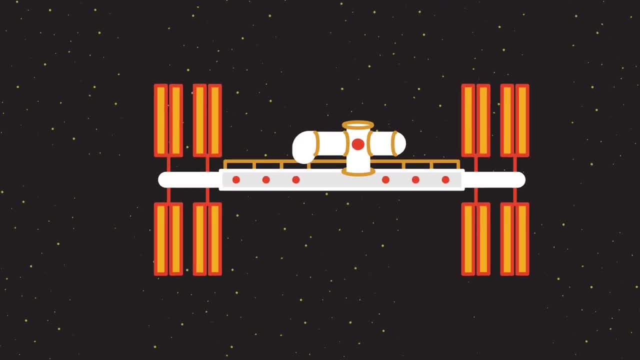 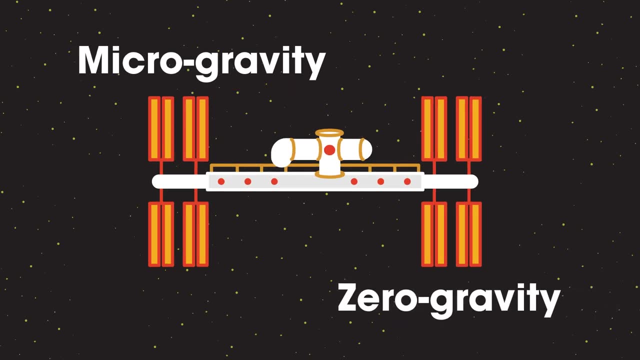 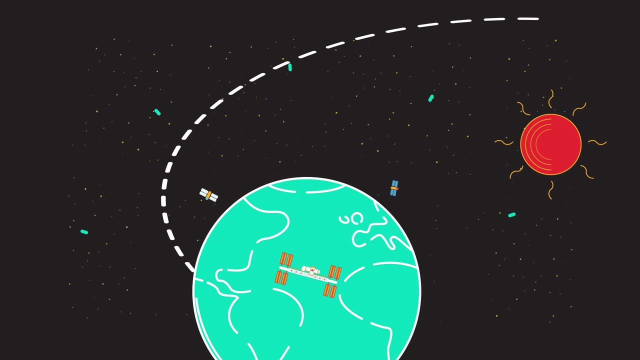 People often explain weightlessness in the space station as caused by the lack of gravity and talk of microgravity or zero gravity. But the space station is orbiting the Earth like the Earth orbits the Sun. It's the gravitational force between the Earth and the space station, so gravity is. 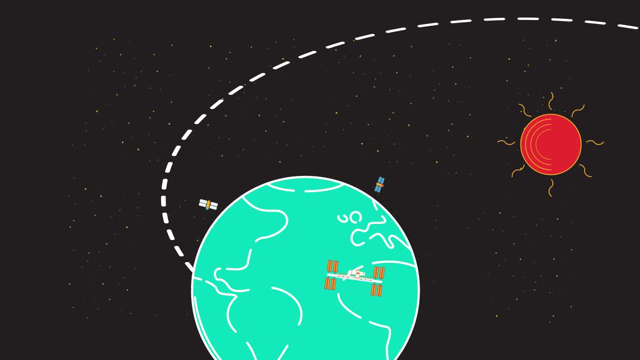 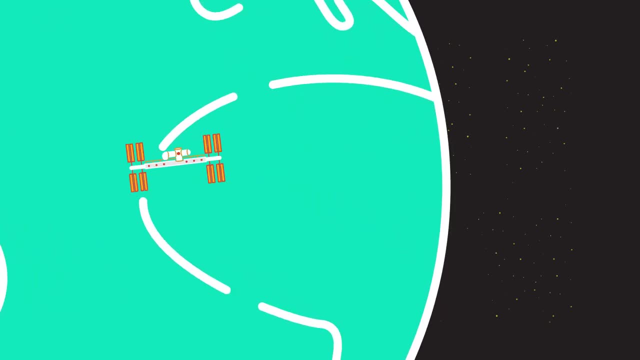 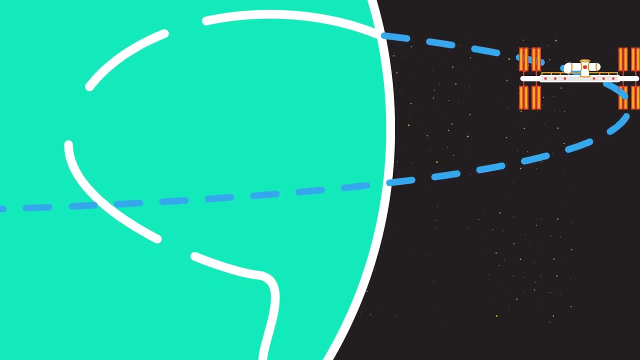 the space station that keeps it, and all the objects in it, in Earth's orbit. If the space station were not moving, it would fall straight down towards the center of the earth In an orbit. it is constantly in a free fall as it constantly bends round in its orbit. All the objects and people in the space